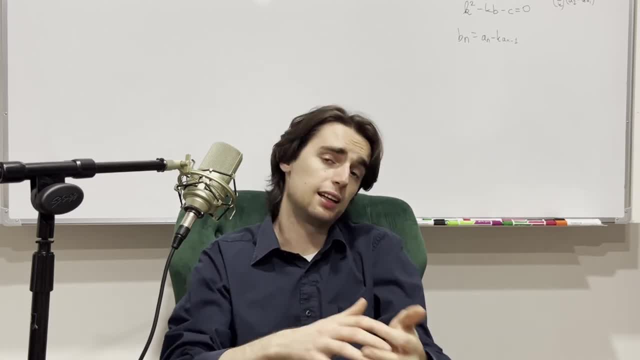 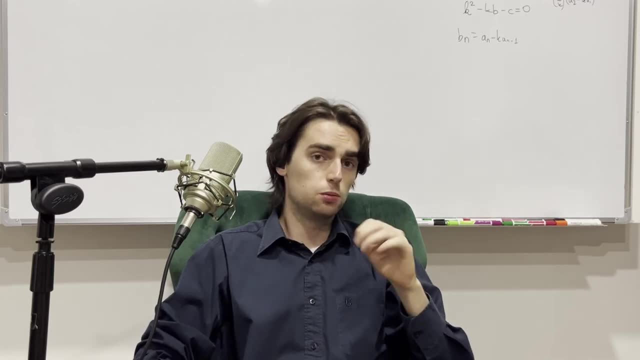 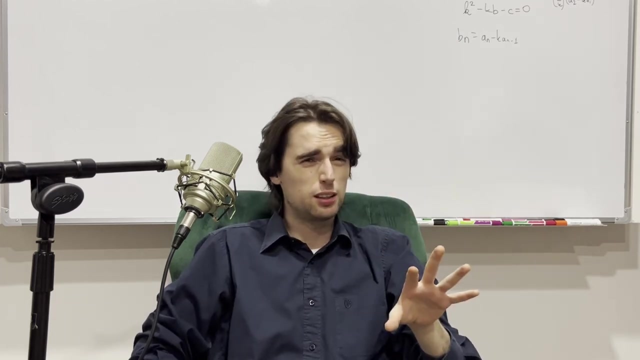 open up the space for you to learn more deeply things about polynomials or even geometry that involves complex numbers. So that is sort of the introductory level. And then you need to learn about induction. Actually, before you learn about induction, you need to also understand quadratic-quadratic equation: what it is, what its solutions are. 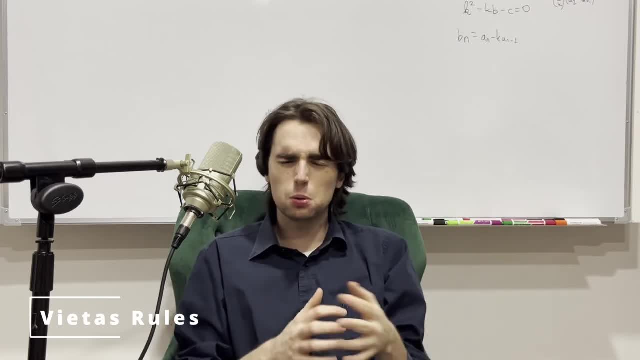 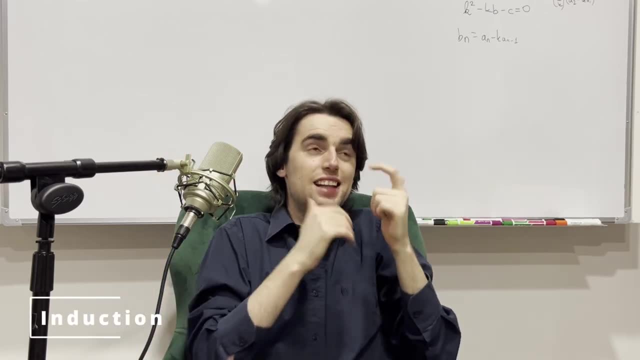 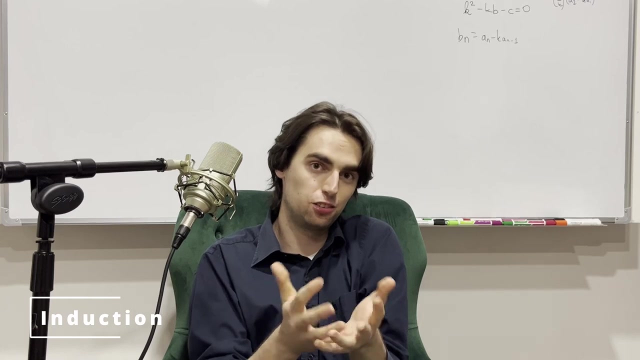 Vieta's rules, And these are things you learn a bit in school. And after you've done the quadratic, then we move on to induction, which is a big thing. It's a next level of thinking that you use often in all fields, But I think it's also very much used in algebra. Say: how do you prove? 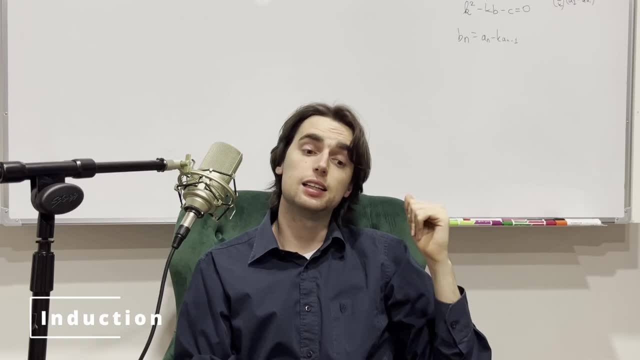 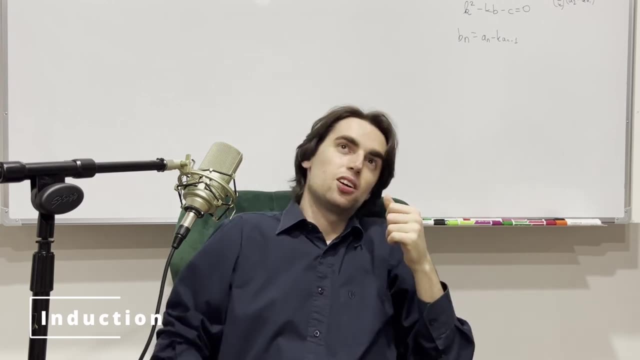 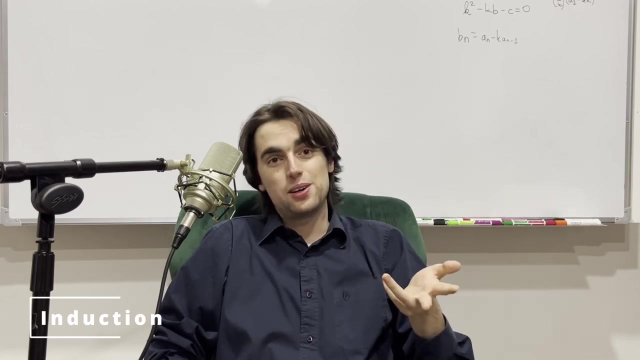 that Two to the power of n is is greater than or less than n factorial. How do you go about doing that? It's less than n factorial. Or say, is two to the n or n squared, which one is greater? 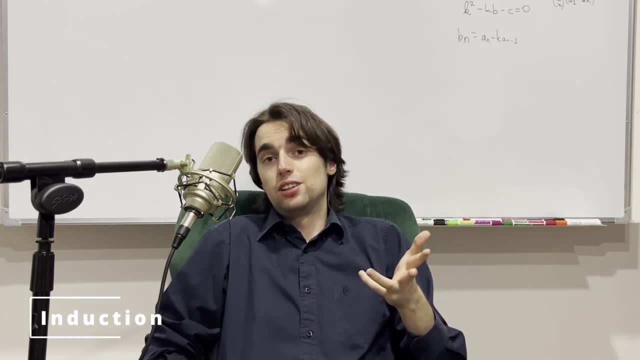 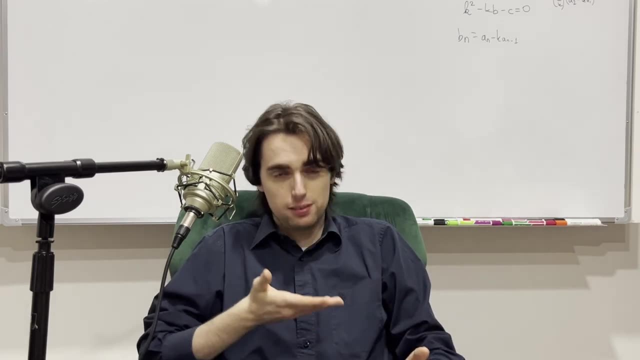 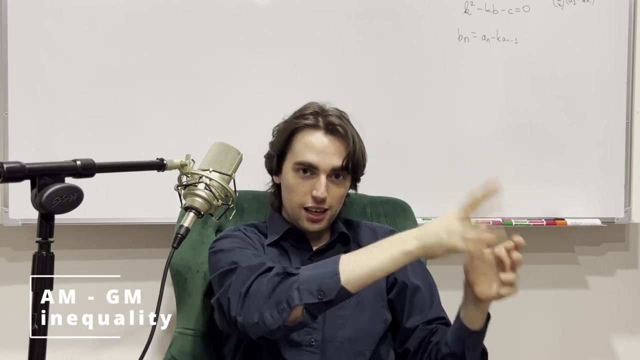 How are you going to prove these things? And induction is the answer to that. Then, after induction, you also want to. after you've done the basics of inequalities, you also want to learn about some more advanced inequalities, like: yes, okay, we start with AMGM, then we learn Cauchy and Schur's inequality. 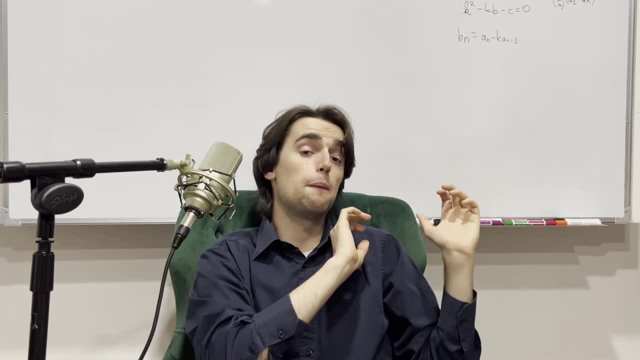 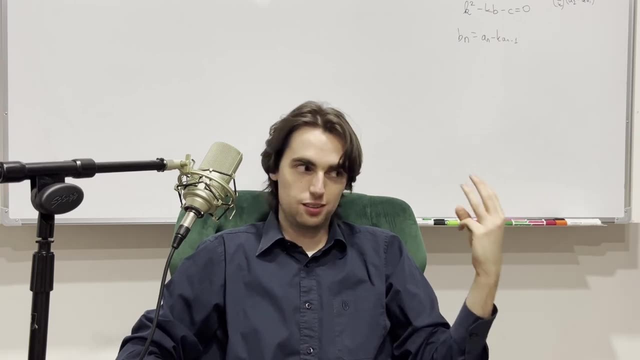 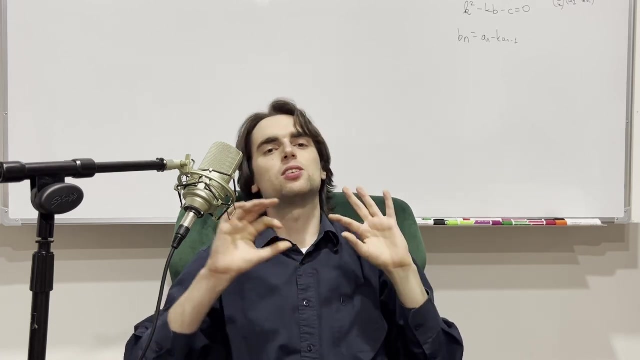 And after that you can really solve a big, big portion- like 80% of all math problems and inequalities with those where you just know those three, the AMGM, Schur and Cauchy. But then you can learn some other things like the rearrangement, inequality. 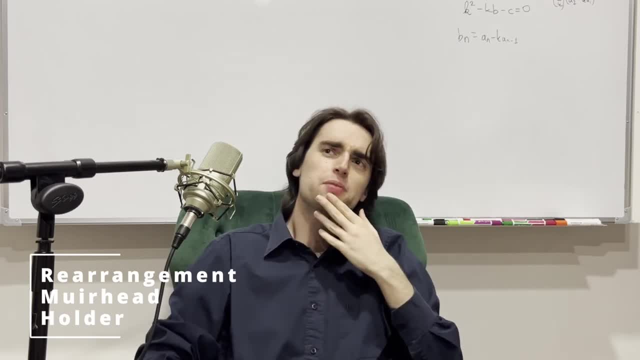 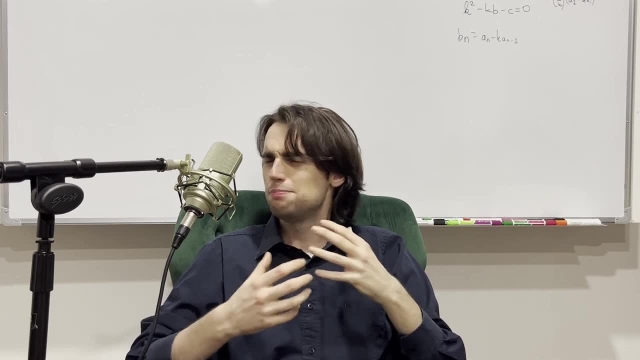 Murrhead, I don't know the exact name- Holder's inequalities like a bit more of a generalization of Cauchy-Schwarz, And there are many other things that you can learn. build up this theory, But really. 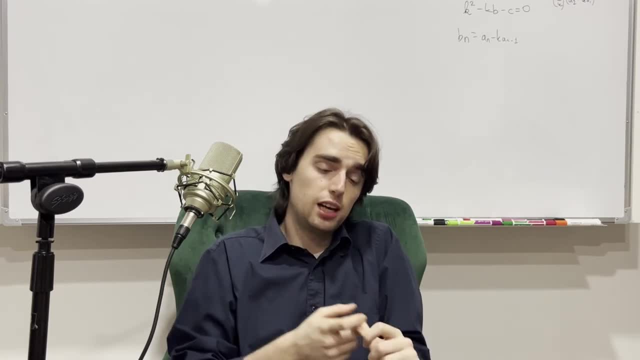 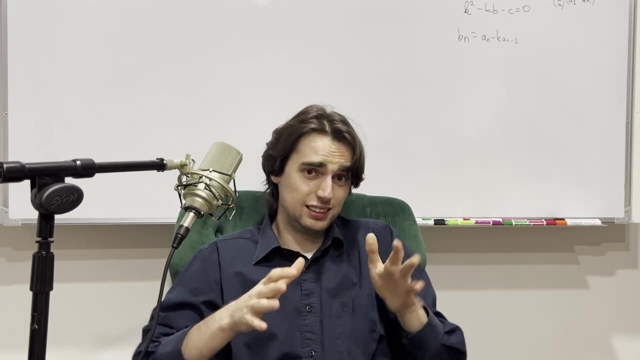 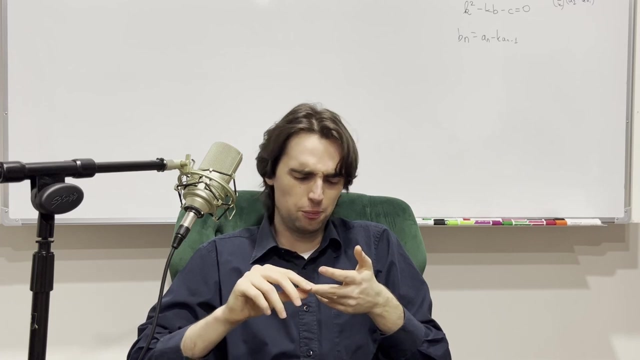 if you know the basics here- and I'm calling the basics AMGM or AMGM- and the quadratic, the power, mean maybe the generalized, is a bit advanced And it's only been used, I believe, once at the IMO. the IMO 2020 problem number two: 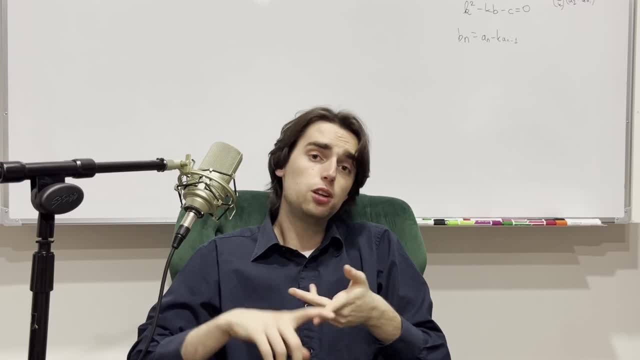 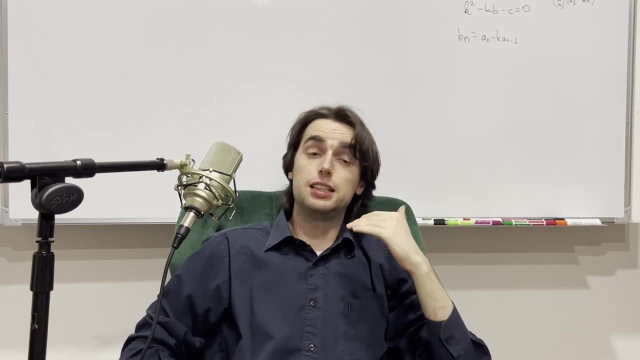 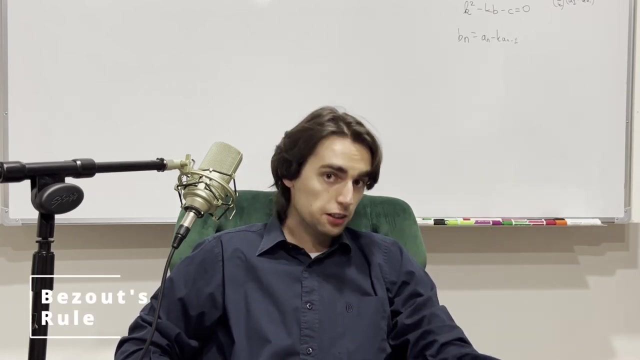 And after that you also have Cauchy and Schur, like these are the basic tools and you build up from there. Then after she also want to dive deeper into polynomials. Yes, you have some rules like: if you have a zero, then you can factor the polynomial. 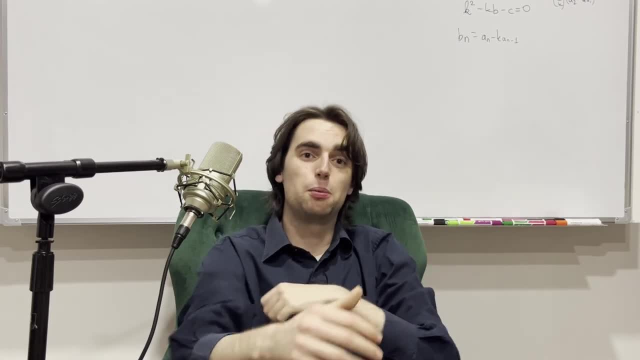 But then there's so much more to learn with polynomials And I'll be making a video series on an introduction to polynomial so you can definitely check that out if you want to learn more about that. But I'm keeping you updated. So that's part one. so I call that a wheelboat. 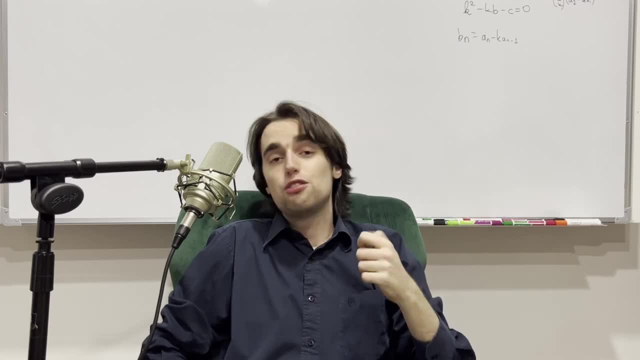 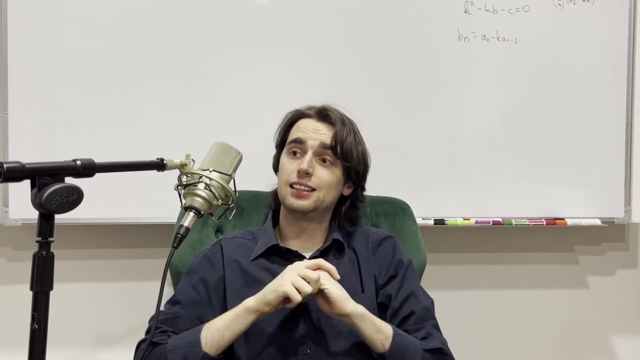 51, 00 JAN, maybe two days before the start of training. one of these them: after polynomials there's also functional equations, like these. things all go hand in hand, right? you learn a bit of polynomials, then you do some functional equations and a subset of. 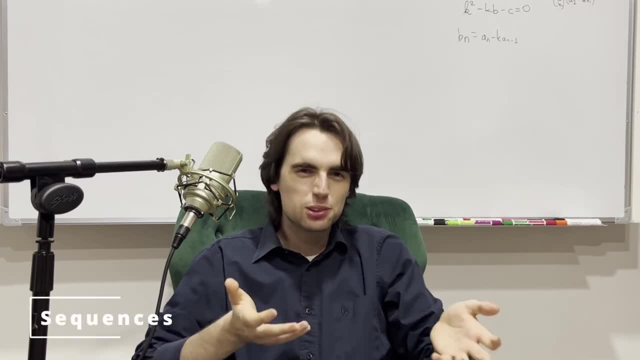 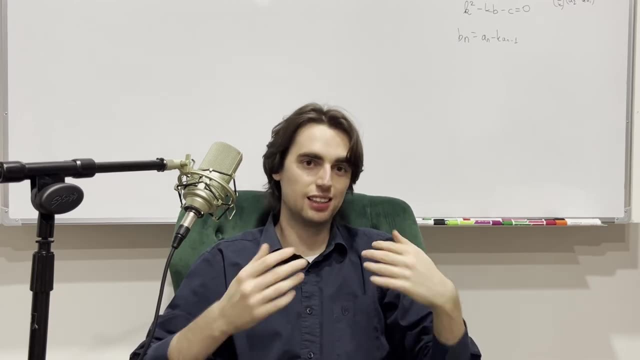 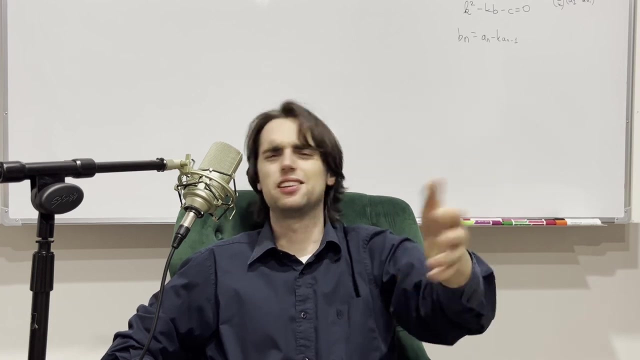 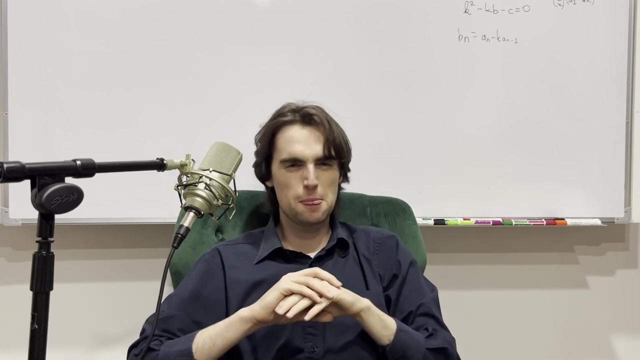 functional equations is sequences which you can also think of, functions from the positive integers or the non-negative integers or the natural numbers to to some other subset, right like real numbers integers, again positives. but that's really what sequences are, and these are beasts of their own sometimes these are like you know, these are functions from n to r. that's a way that you can. 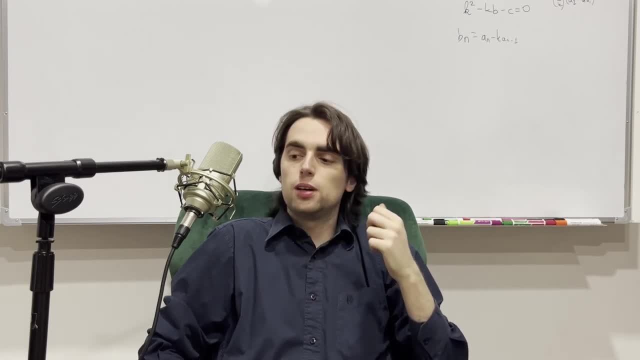 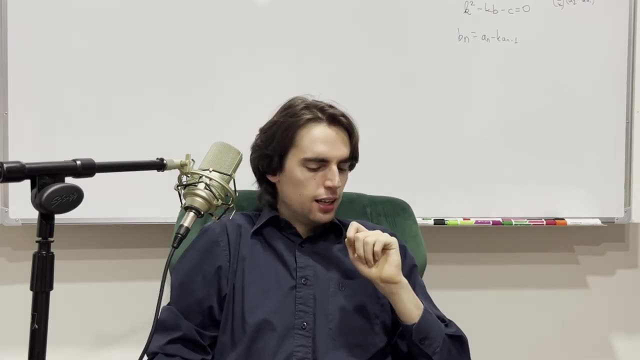 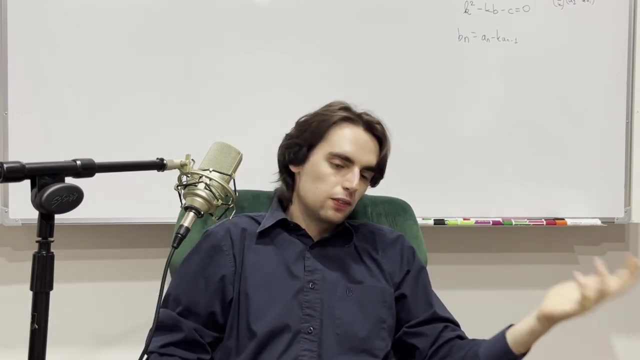 also look at sequences. that's the thing to know. we've covered reata's rules and with that. am i missing anything? and the final thing that i actually forgot is how to do recursive equation, how to solve them. there's also things with equations like arithmetic and geometric series. 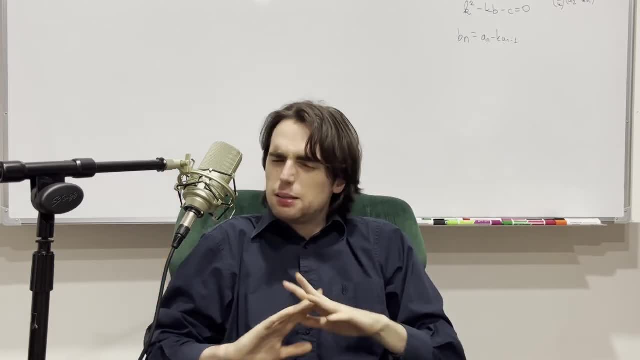 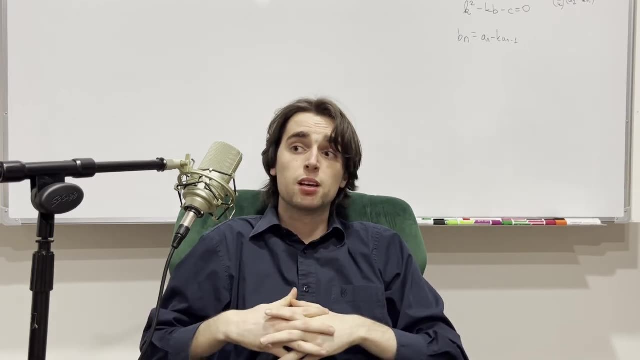 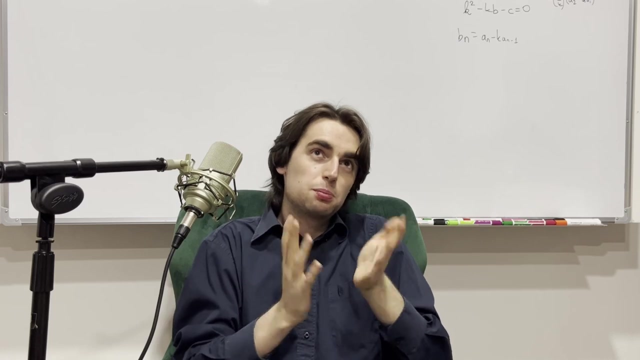 and maybe, maybe- though this is not by any means necessary, at least not now, at the making of this video wasn't necessarily the IMO when I came to the IMO, but maybe just like the basics of understanding of what, how, that calculus per se, though that can be helpful, but maybe 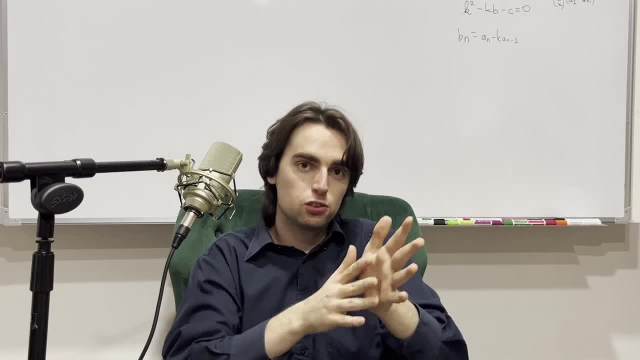 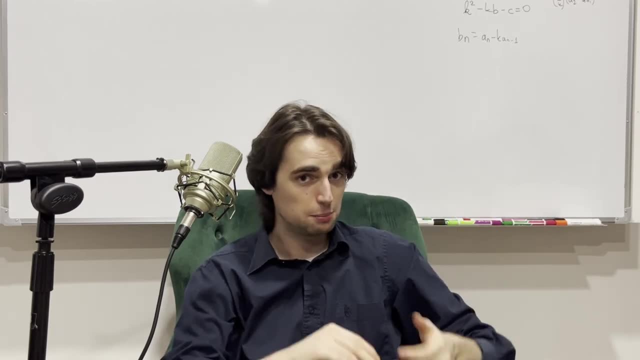 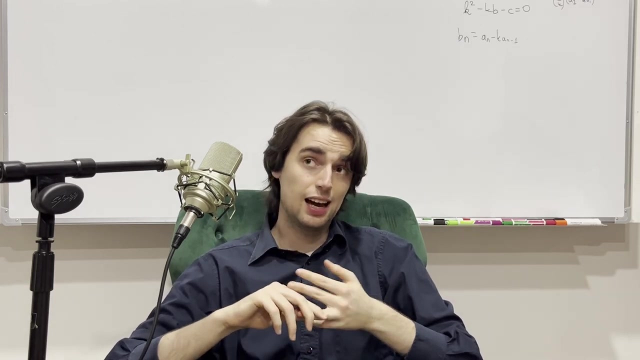 and this is really- I want to stress this very much. so for those of you that are just about, I want to learn so much theory, theory, theory. you don't really need that much if you just learn the basics of induction, so also functional equations, the three basic inequalities, and with